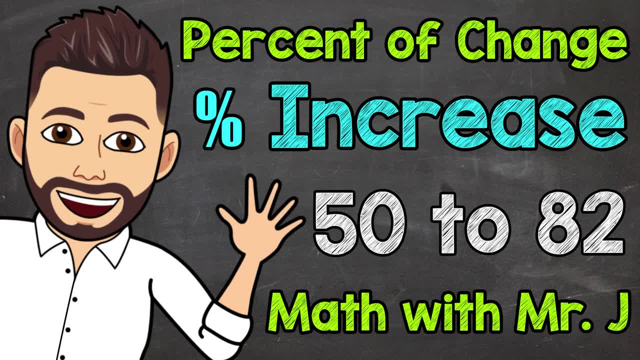 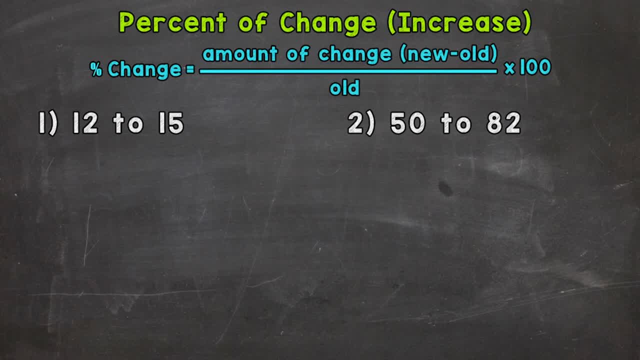 Welcome to Math with Mr J. In this video I'm going to cover percent of change and, specifically, percentage increase. We have two examples that we're going to go through together in order to get this down. Now, when we calculate a percent of change, we need to take the amount of change. 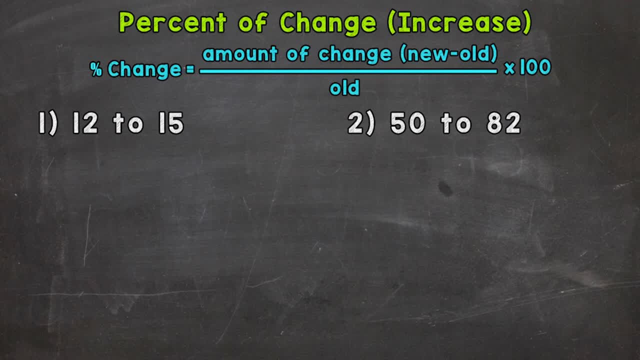 so the new number minus the old number and then divide by the old number. We lastly multiply by 100. So when we do the amount of change divided by the old number, we're going to get a decimal. We multiply by 100 to convert that decimal to a percent. 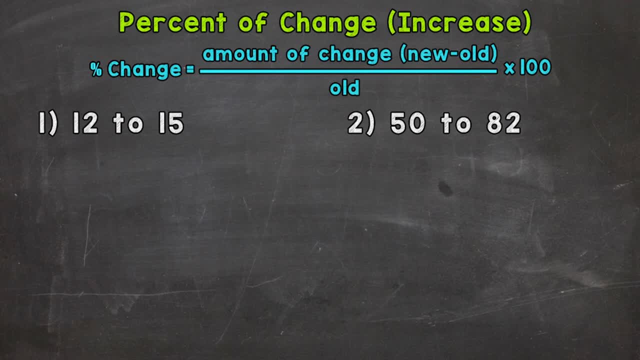 Let's jump into number one, where we have 12 to 15.. So we start with a 12, and now we have a 15. So we can see that we had an increase. So let's plug our numbers in to our formula to calculate percent of change. 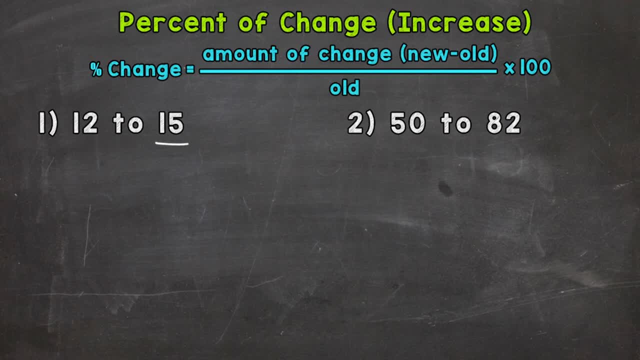 So we need to take the new number, which is 15, and subtract the old, So 15 minus 12 gives us an amount of change of 3. We need to divide by the old number, so the old or original number is 12, and then multiply by 100. 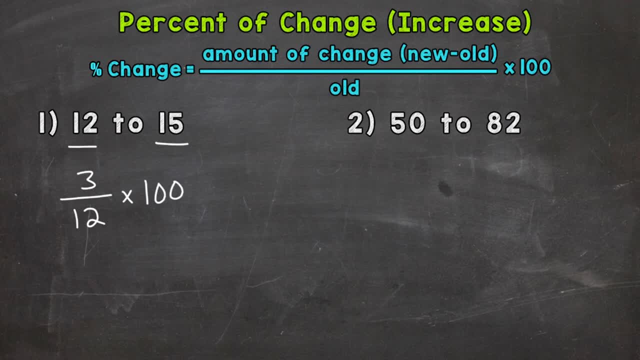 Now I do want to mention that it's very important to always divide by the old or original number, because that's the number that changed. We want the percentage change relative to the number we started with. We are looking at the percent that that number changed. All right, so 3 divided by 12,. 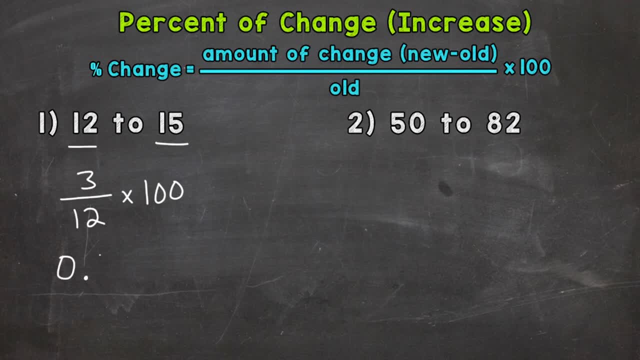 that's going to give us 0.25.. We need to multiply that by 100 in order to convert it to a percent, So we can move the decimal twice to the right when multiplying a decimal by 100.. So 1,, 2,. 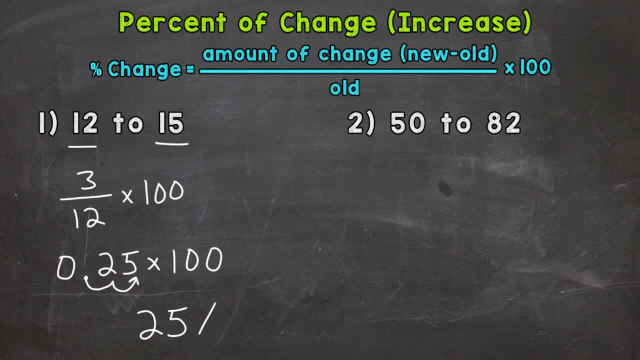 and we end up with 25%. So we had a 25% increase, 25% increase. And that's our final answer for number one. Let's try another one and move on to number two, where we have 50.. So we start.